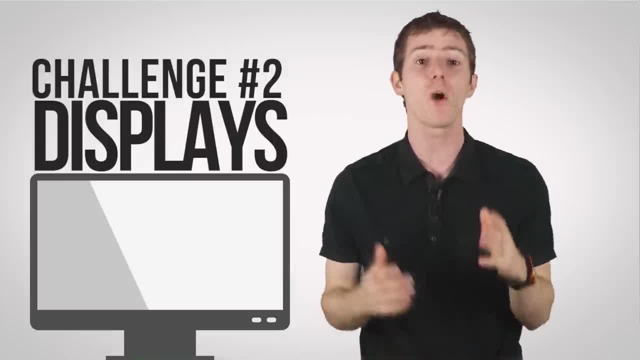 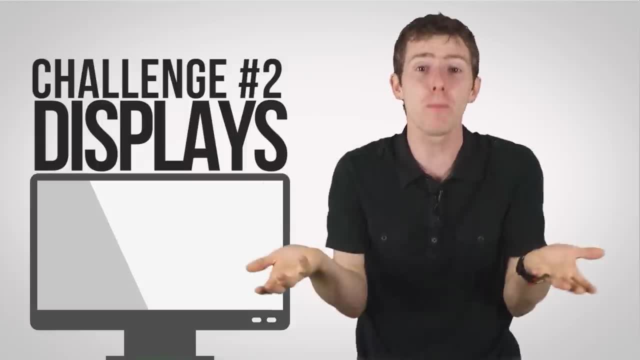 Let's say you pony up for a Blu-ray of your favorite movie and then watch it on a cheap TV or TN panel monitor. In this case the data is all there, but your display is not capable of reproducing all those colors. 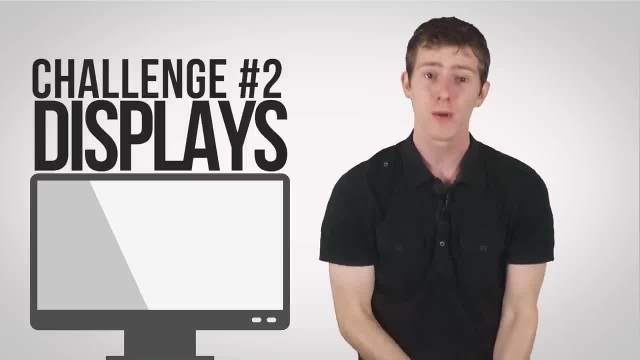 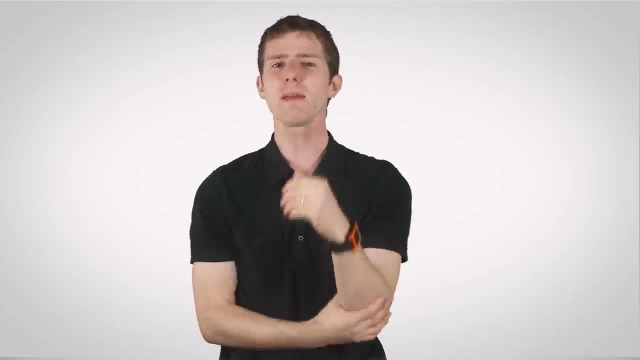 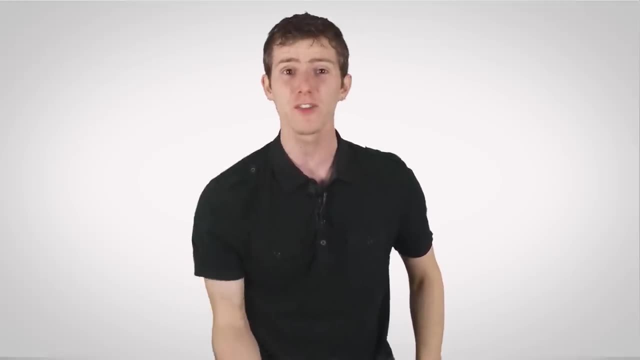 so you'll see the same blockiness and color banding as before, where the display is just approximating the color as best it can. Alright, so let me get this straight, Linus: You're telling me that my viewing experience sucks when I was perfectly happy with it before, and then you're following up by telling me that there's basically nothing I can do about it. 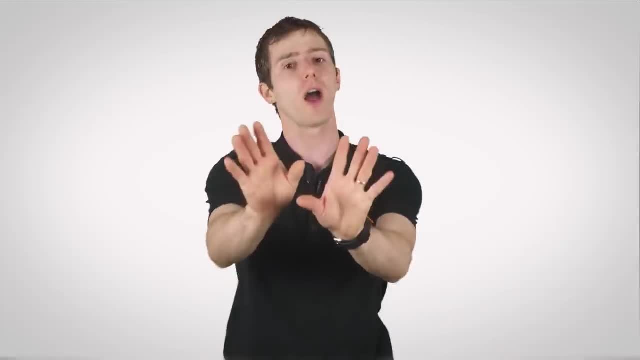 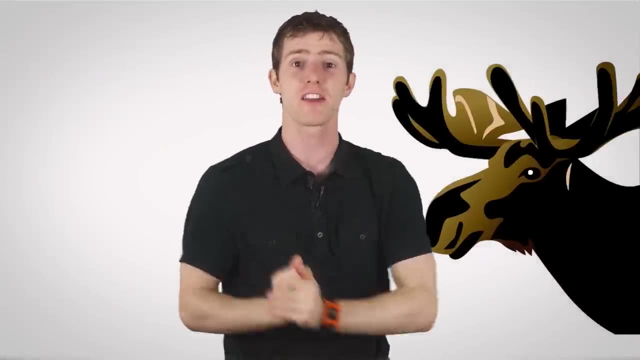 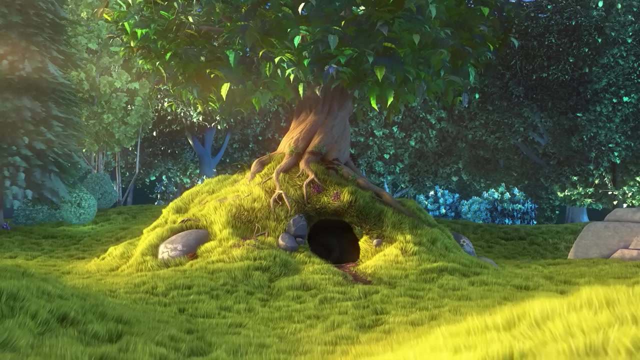 without spending a bunch of money anyway. Are you just trying to make me unhappy? No, I'm not. I know all of this and I'm still perfectly happy in. you know Canada here with my Canadian internet connection and you know Canadian Netflix. It especially doesn't bother me on small screens like on a phone or a tablet, and in 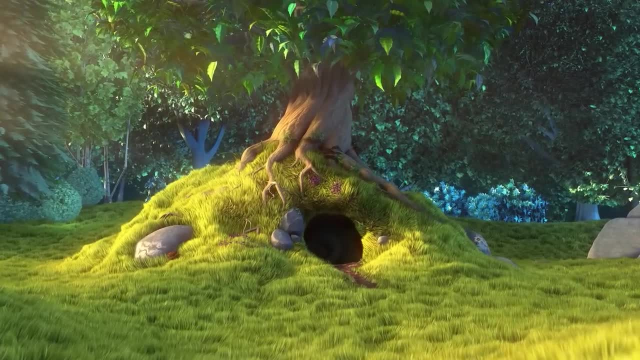 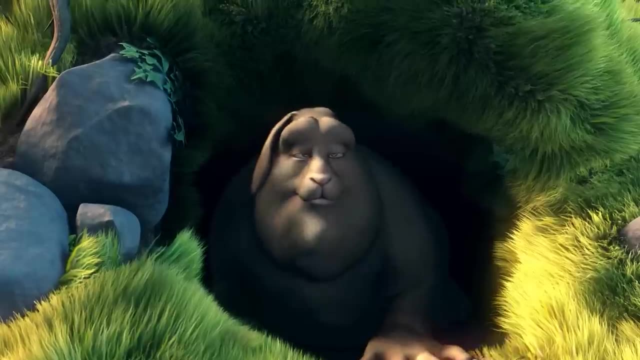 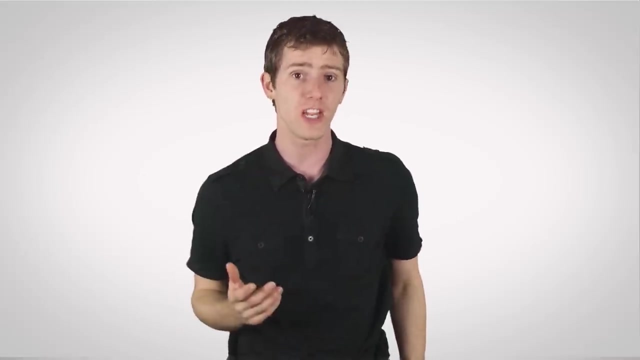 vibrant scenes with many varied colors. It only really bugs me in dark scenes with many similar colors. I mean, see that right there. The blockiness and lack of detail on the bunny when he's covered by the shadows is a perfect example of what we're talking about. And just because we're aware of this and understand it better doesn't mean we have to change anything. 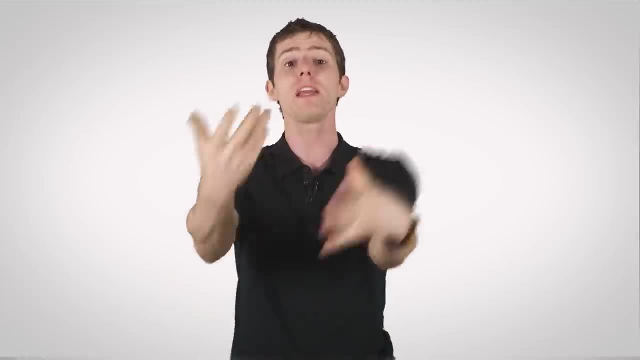 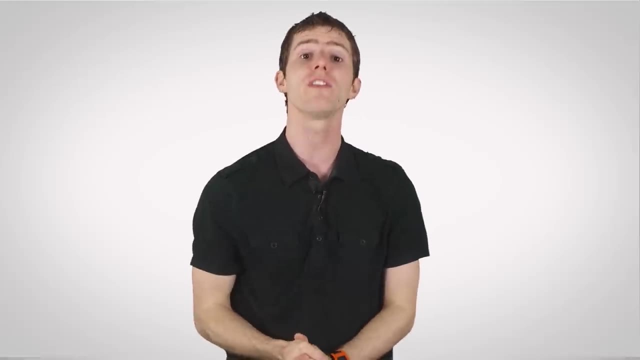 I've just wanted to cover this topic for a while, so that I can explain to folks why their HD image doesn't always look that great. That way, if they do want to do something about it, they'll know what to do. Look for content that uses high quality codecs and is encoded at higher bit rates. 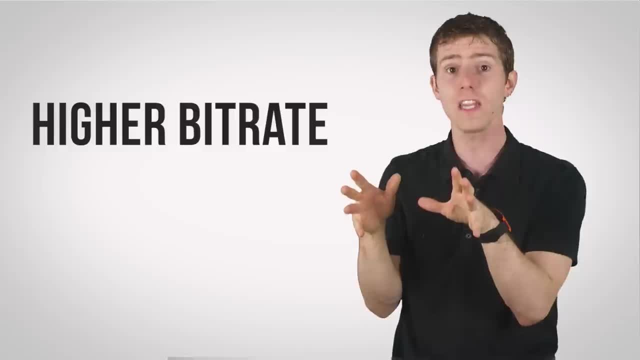 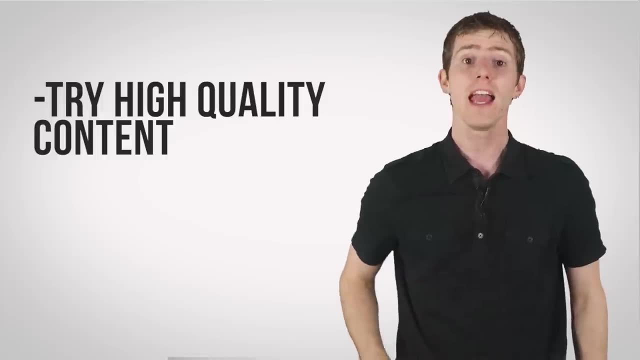 The higher the bit rate or the amount of data per second in the video stream, the higher the color depth is likely to be. Try higher quality content first before upgrading your display, and use shadows as a quick and easy benchmark to see if it's making a noticeable difference. 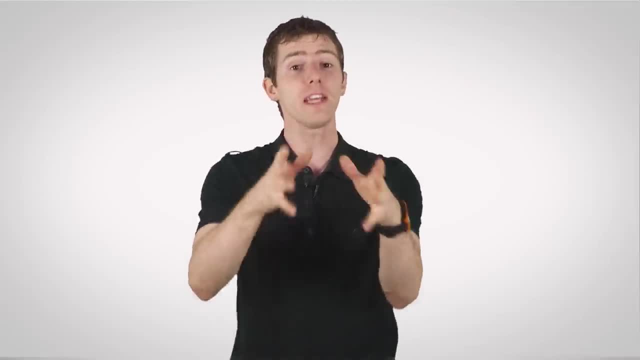 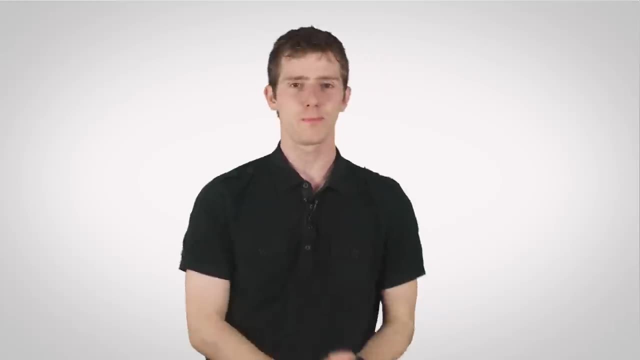 And if it doesn't make a difference to you, then that's great, because there is a limit to what your eyes can see anyway before more color depth really doesn't make a difference anyhow. Speaking of shadows, our featured audiobook from audiblecom today is: 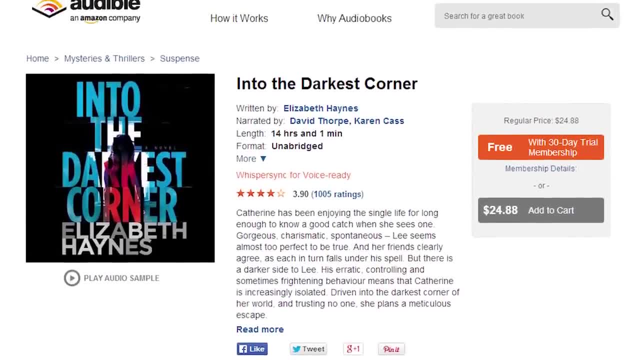 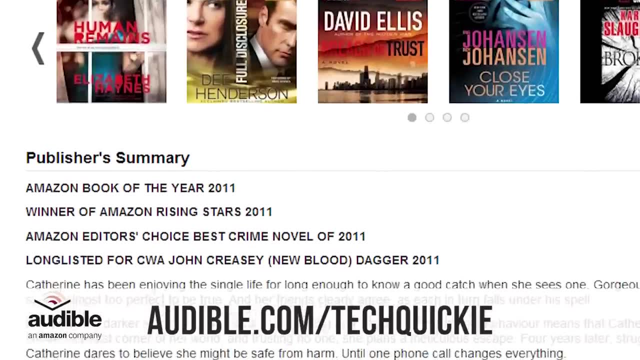 Into the Darkest Corner by Elizabeth Haynes. You can get it or something else for free by going to audiblecom slash tech quickie linked in the video description and signing up for a new account. It's an editor's pick on audible. It won Amazon's Book of the Year award in 2011,.